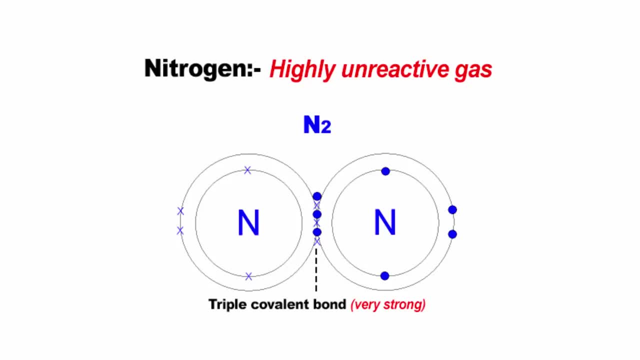 of energy required to break the bond between two atoms which have triple covalent bonds is incredibly high. The more energy required, the stronger the bond is said to be. In a nutshell, triple bonds are difficult to break Because they require a lot of energy to break. 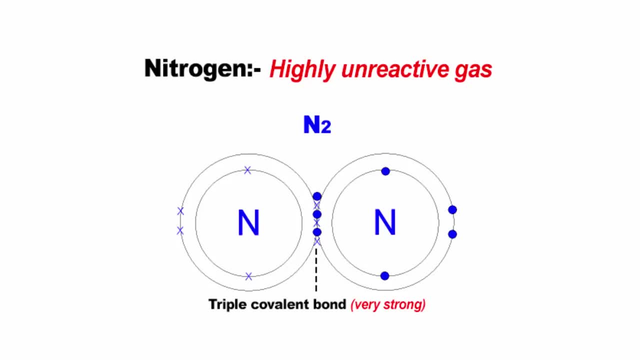 Now nitrogen molecules have a triple bond And that makes it very unreactive Because it requires a huge amount of energy to break the bonds. Now the big question is: where are you going to find that kind of energy? Once the strong triple bond is broken, nitrogen atoms are very reactive, So the whole meaning 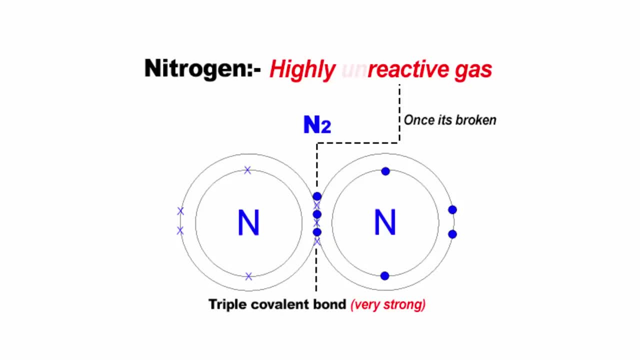 of the nitrogen cycle is to break the nitrogen molecules so that it can be utilised by plants and animals. Now the question is: how do we break the bonds, How to break the nitrogen molecule? Turns out there is a solution to that. There has to be a way by which nitrogen gas in the 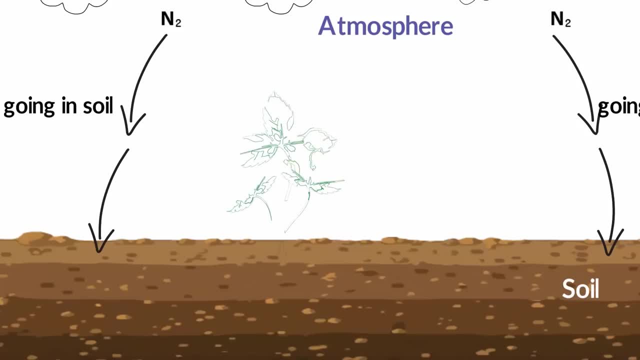 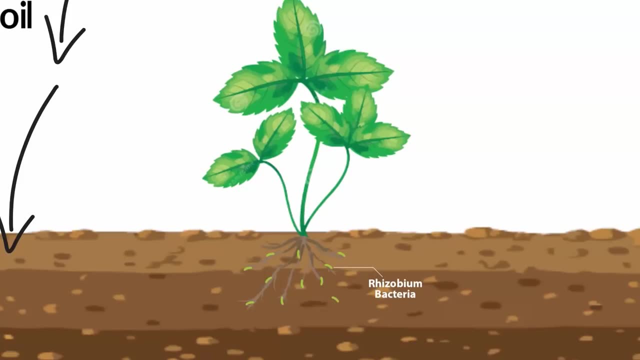 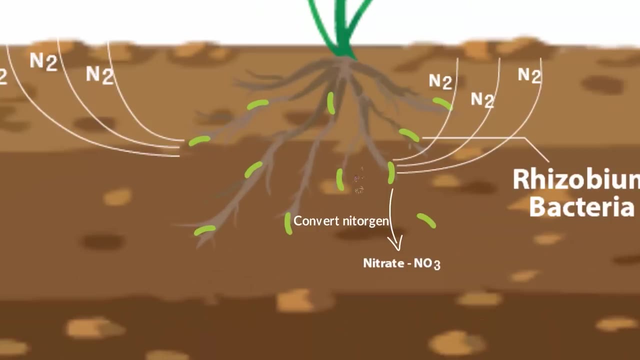 atmosphere must find its way into the soil. This is where bacteria in the soil comes into the picture. The roots of these plants are colonised by rhizobium bacteria. These bacteria have the ability to directly convert nitrogen into useful nitrogen compounds with the use of. 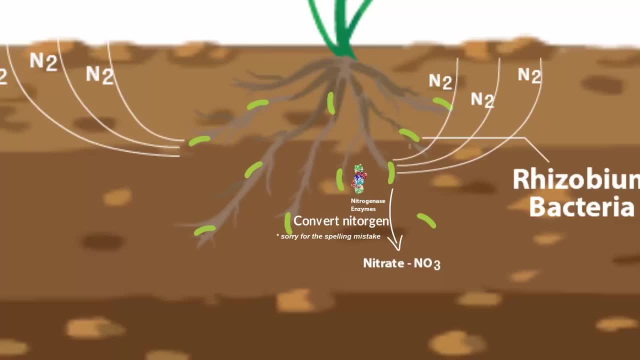 a special enzyme called nitrogenase. This enzyme is known as nitrogenase. In other words, rhizobium bacteria carry the nitrogen from the air to the soil and transform into another form called nitrates. This process is called nitrogen fixation. Just remember: nitrogen fixation takes unreactive nitrogen from the air and turns into a usable 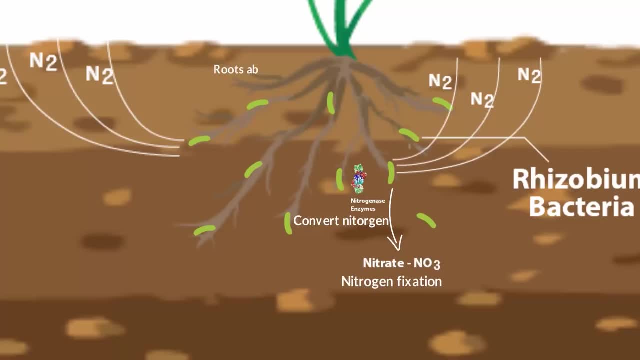 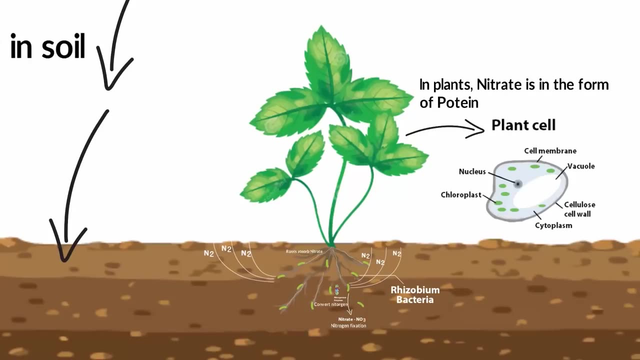 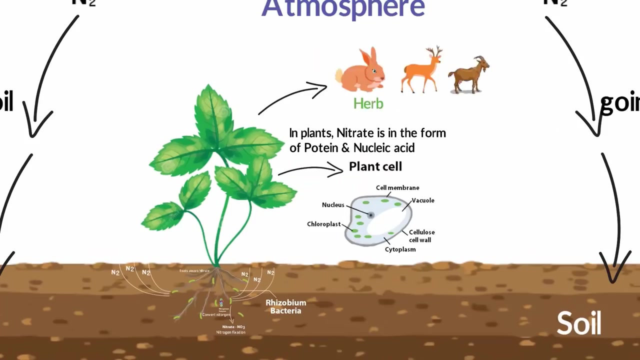 form After nitrogen fixation. roots of plants absorb the nitrate In the plant. they are in the form of protein and nucleic acids. If you can recollect the ecological pyramid in that we have seen that plants are producers and herbivorous animals feed on plants for food and energy. 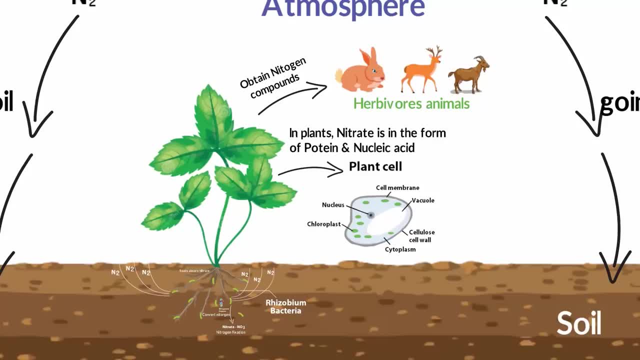 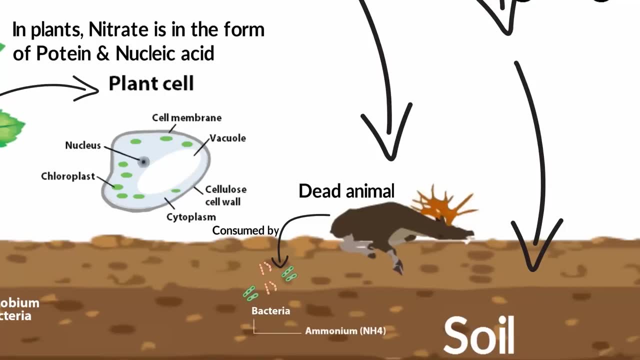 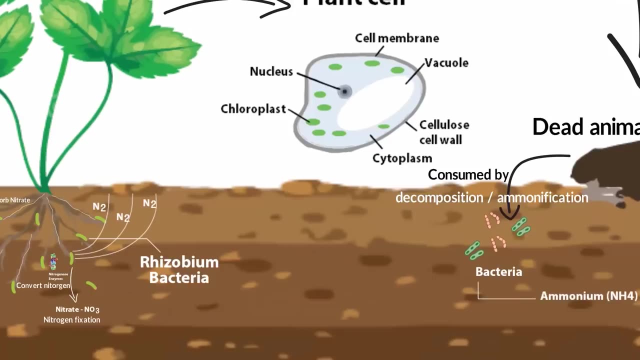 That's how animals get the nitrogen they need: by eating plants. When animals produce waste or die, bacteria consumes this dead organic matter. As a result, the nitrogen in this waste is in the form of ammonium. This process is called decomposition or ammonification.